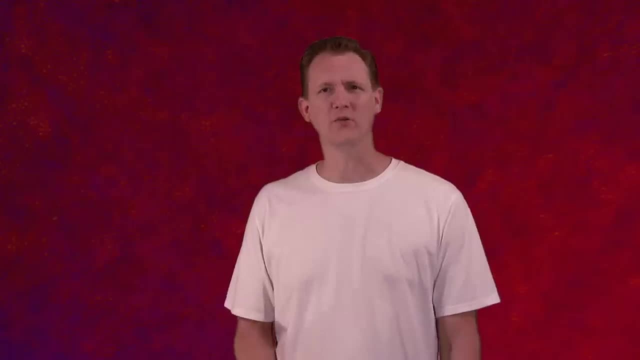 or unlike fractions, And we learned that the only way we can do that is to change our fractions so that they do have the same bottom number. Alright, then how do we do that? How can we change two unlike fractions into two like fractions? How do we get our fractions to? 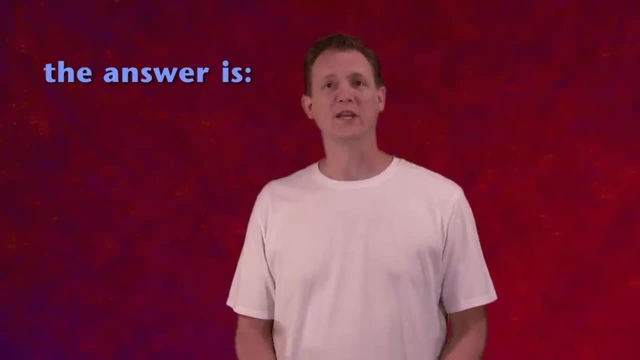 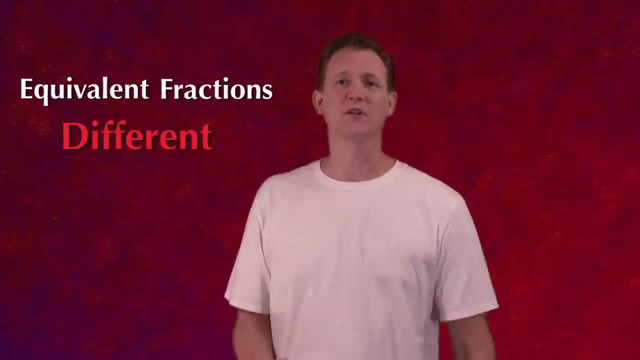 have a common denominator. The answer is we need to use equivalent fractions. You remember what equivalent fractions are? right, They're fractions that have the same value but use different top and bottom numbers, like 1 over 2 and 2 over 4. They both represent one half. 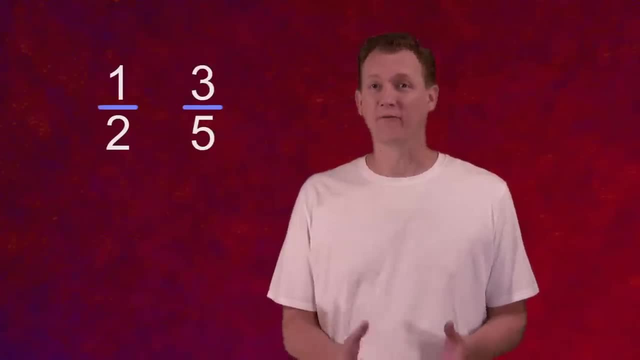 but with different numbers. Well, whenever we have two unlike fractions that we need to add, if we could find equivalent fractions to use instead and if those new equivalent fractions had the same bottom numbers as each other, then we'd be all set. We'd have two like fractions and we could add them. 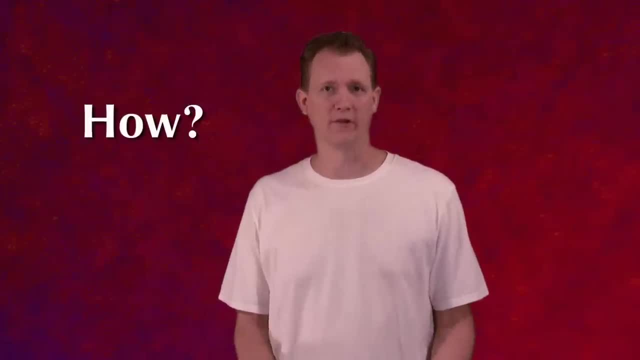 using our procedure. Okay, but how do we find equivalent fractions that have a common denominator or the same bottom number? Well, there's two main ways of doing it. In this video, we're only going to learn the first way of doing it, And I like to call this way finding the easiest. 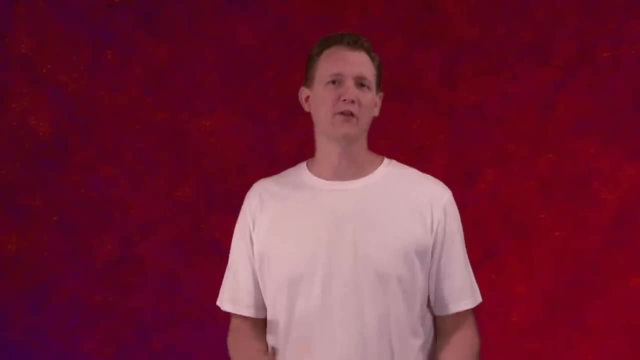 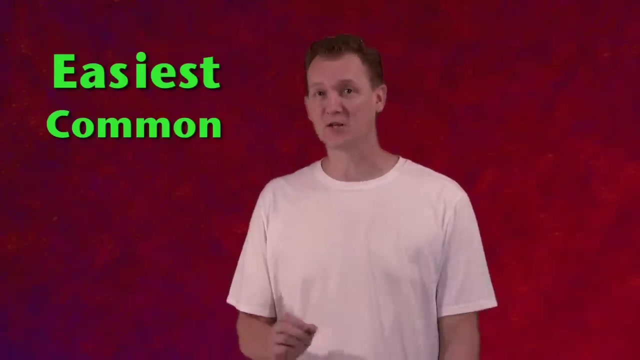 common denominator. In the next video, we'll talk about another method that some of you may have already heard about. It's called finding the least common denominator. Okay, so how does this easiest common denominator method work? Well, even though this is an easy, 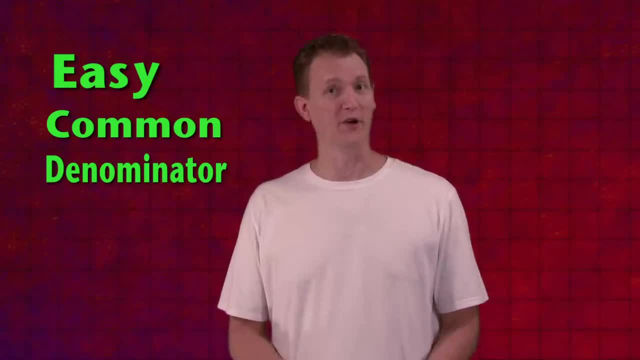 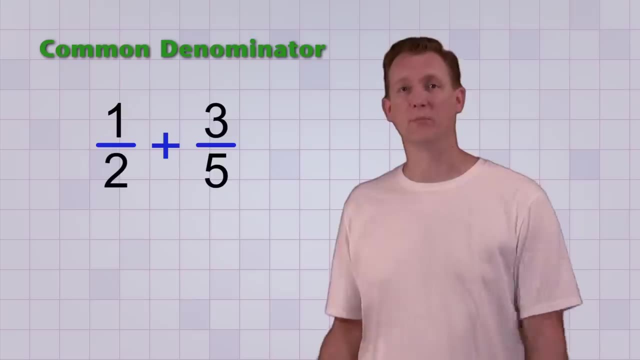 method. it might sound a little complicated at first, But don't worry, it'll make a lot more sense once you've seen a few examples. In this method, the common denominator is always going to be the product of the bottom numbers. In other words, it will be the number you'd get if you multiplied the bottom 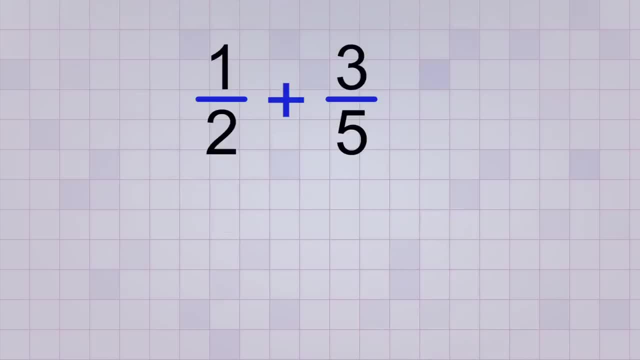 numbers together. Basically, all we're going to do is take the two different bottom numbers and make two different whole fractions using them. Then we're going to move the whole fractions to the opposite sides and multiply them by our unlike fractions. Doing this will give. 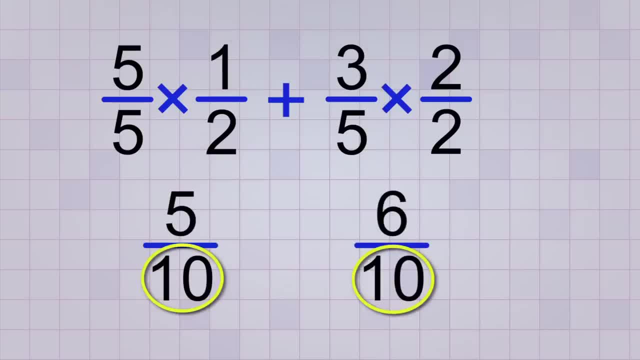 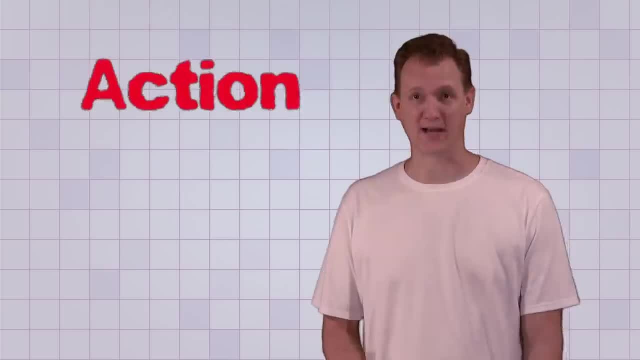 us two new equivalent fractions that will have the same bottom number. Then we can add or subtract them easily. Okay, let's try a couple examples so we can see this method in action. Let's add the fractions 2 over 5 and 1 over 3.. 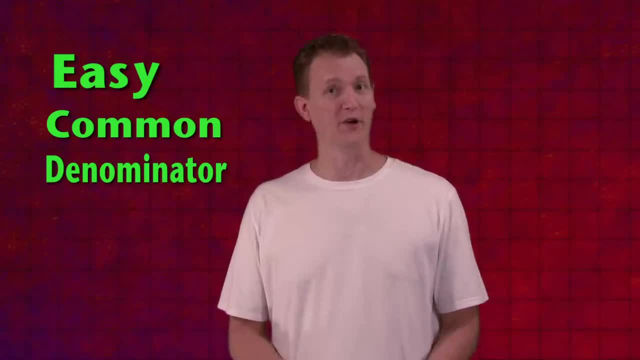 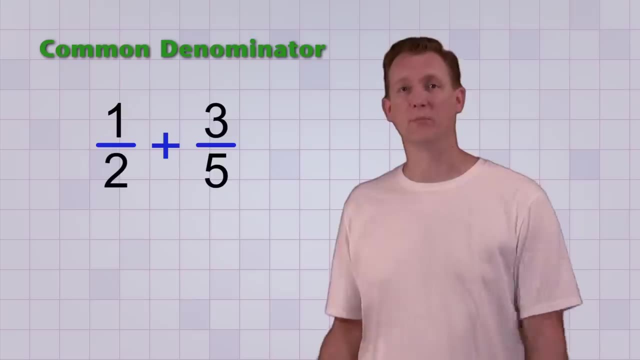 method. it might sound a little complicated at first, But don't worry, it'll make a lot more sense once you've seen a few examples. In this method, the common denominator is always going to be the product of the bottom numbers. In other words, it will be the number you'd get if you multiplied the bottom 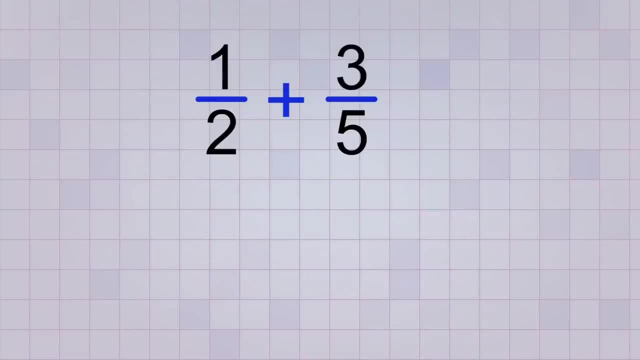 numbers together. Basically, all we're going to do is take the two different bottom numbers and make two different whole fractions using them. Then we're going to move the whole fractions to the opposite sides and multiply them by our unlike fractions. Doing this will give. 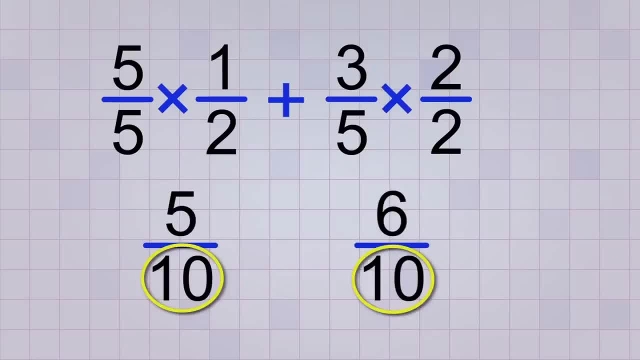 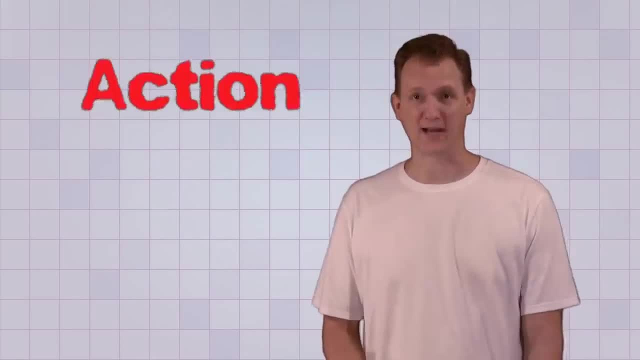 us two new equivalent fractions that will have the same bottom number. Then we can add or subtract them easily. Okay, let's try a couple examples so we can see this method in action. Let's add the fractions 2 over 5 and 1 over 3.. 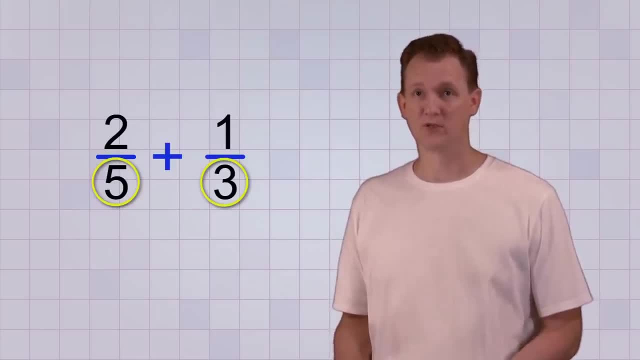 These are not like fractions, because they have different bottom numbers, so we're going to change them, And the common denominator we will use is the product of the bottom numbers. 5 times 3 equals 15.. We change them by multiplying each fraction by a whole fraction. The first whole fraction 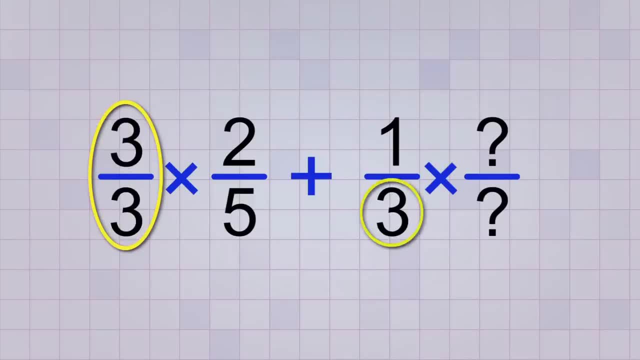 is going to be 3 over 3 because 3 is the second fraction's denominator, And the second whole fraction is going to be 5 over 5 because 5 is the first fraction's denominator. Next we multiply, starting with our first fraction. On the top, 3 times 2 equals 6.. And on the 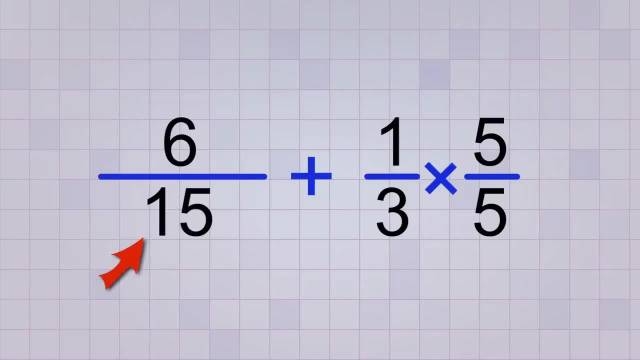 bottom, 3 times 5 equals 15.. So our first fraction has become 6 over 15.. Now for the second fraction: On the top, 1 times 5 equals 5.. And on the bottom, 3 times 5 equals 15.. So our second fraction has become 5 over 15.. 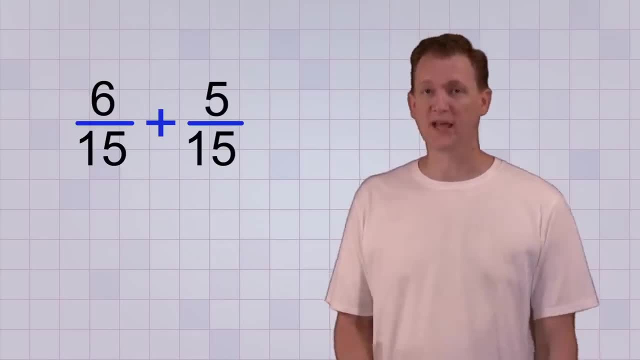 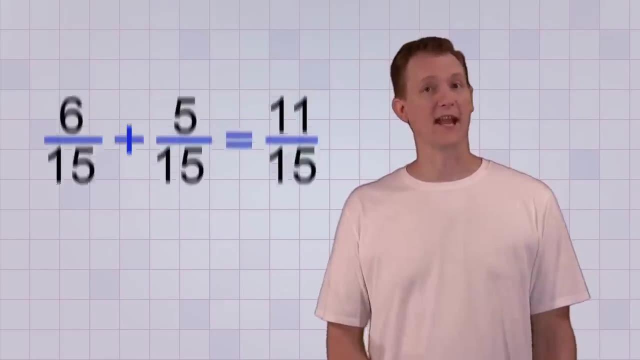 Now we just add them using our procedure for adding like fractions. We add the top numbers: 6 plus 5 equals 11. And then we keep the same bottom number, which is 15.. So that means the answer to 2 over. 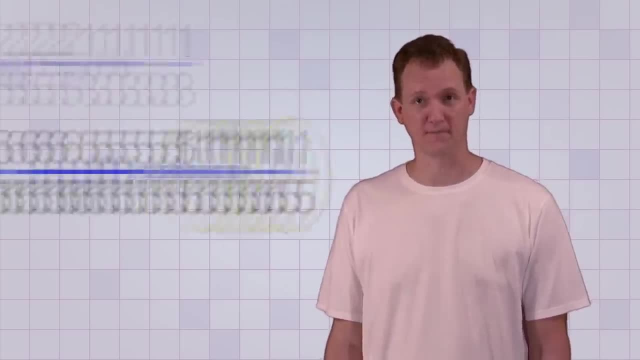 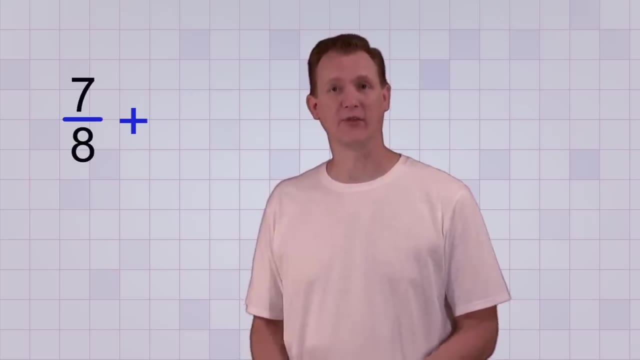 5 plus 1 over 3 is 11 over 15.. That's pretty easy, huh? Alright, let's see one more example of this method. Let's add the fractions 7 over 8 and 3 over 10.. 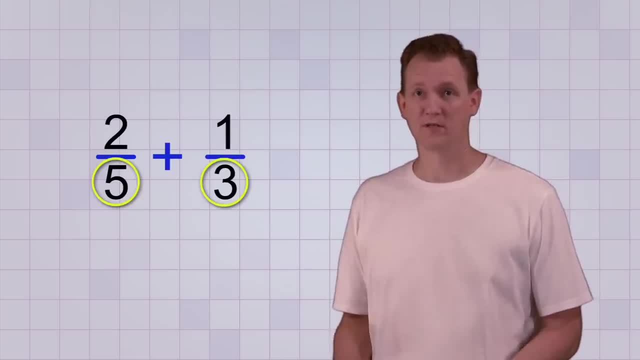 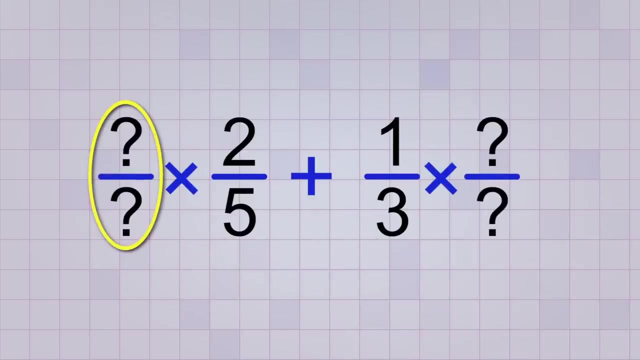 These are not like fractions, because they have different bottom numbers, so we're going to change them, And the common denominator we will use is the product of the bottom numbers. 5 times 3 equals 15.. We change them by multiplying each fraction by a whole fraction. The first whole fraction 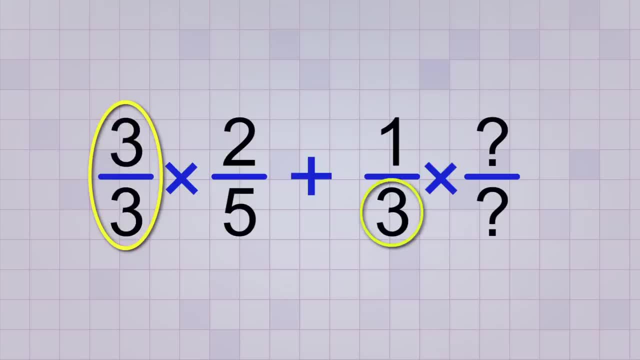 is going to be 3 over 3 because 3 is the second fraction's denominator, And the second whole fraction is going to be 5 over 5 because 5 is the first fraction's denominator. Next we multiply, starting with our first fraction. On the top, 3 times 2 equals 6.. And on the 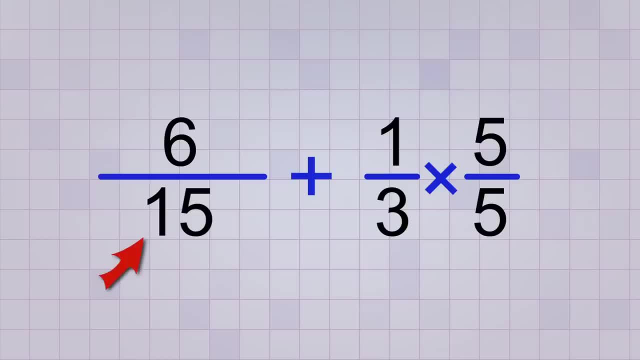 bottom, 3 times 5 equals 15.. So our first fraction has become 6 over 15.. Now for the second fraction: On the top, 1 times 5 equals 5.. And on the bottom, 3 times 5 equals 15.. So our second fraction has become 5 over 15.. 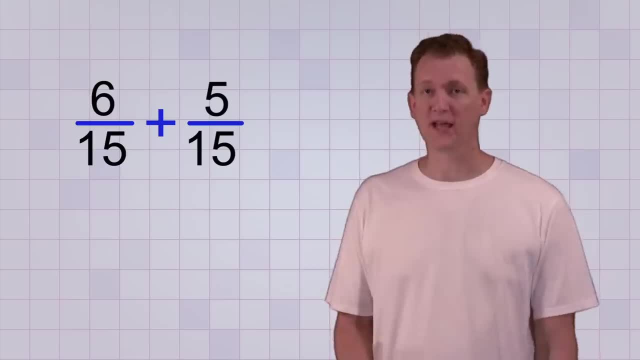 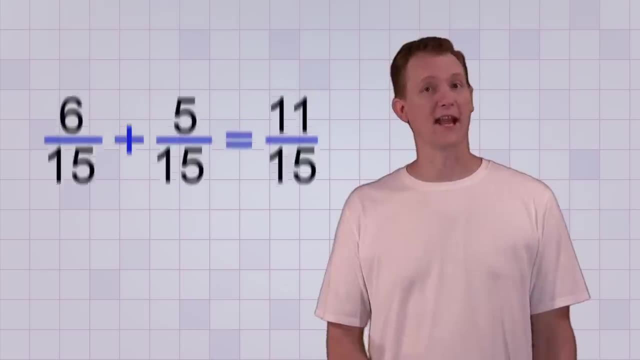 Now we just add them using our procedure for adding like fractions. We add the top numbers: 6 plus 5 equals 15. And then we keep the same bottom number, which is 15. So that means the answer to 2 over. 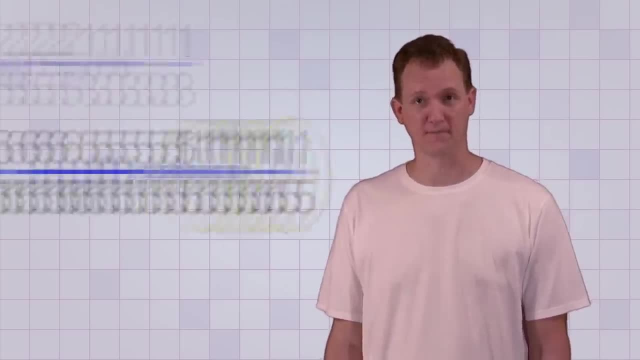 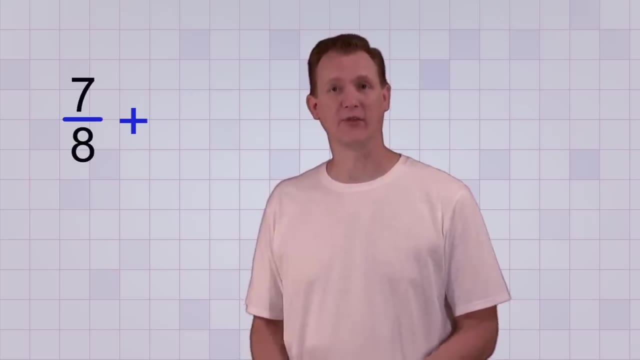 5 plus 1 over 3 is 11 over 15.. That's pretty easy, huh? Alright, let's see one more example of this method. Let's add the fractions 7 over 8 and 3 over 10.. 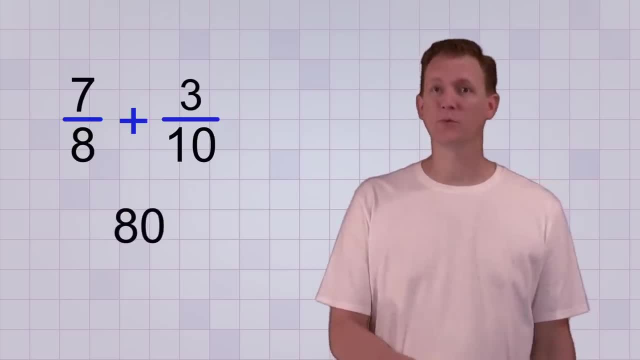 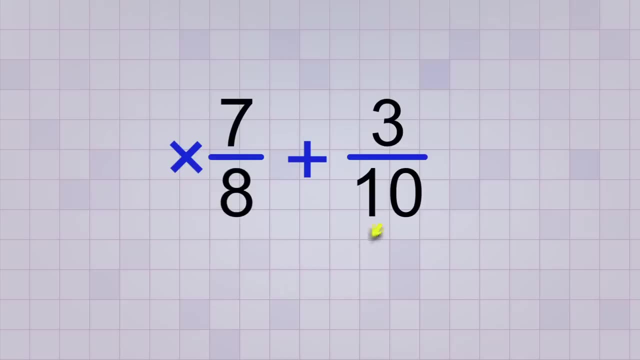 Our common denominator for this problem is going to be 80, because that's what we get when we multiply the denominators together. 8 times 10 equals 80.. We'll multiply our 7 over 8 by the whole fraction 10 over 8.. 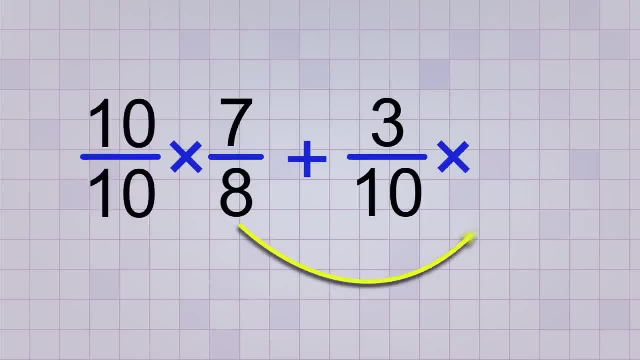 And we'll multiply our 3 over 10 by the whole fraction 8 over 8.. Then when we do our multiplication, the 8 times 10 will give us 80 on the bottom of both fractions. For the top of the first fraction we have, 7 times 10 equals 70.. 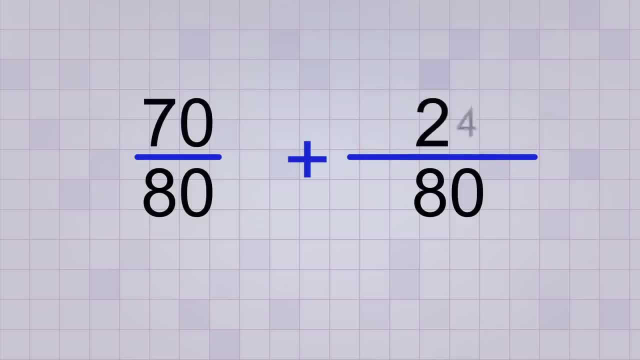 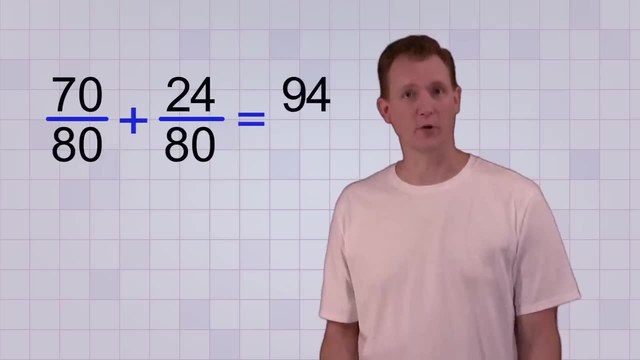 And the top of the second fraction we have, 3 times 8 equals 24.. Now that we have like fractions, we can just add the top numbers: 70 plus 24 equals 94. And keep the bottom number the same: 80.. 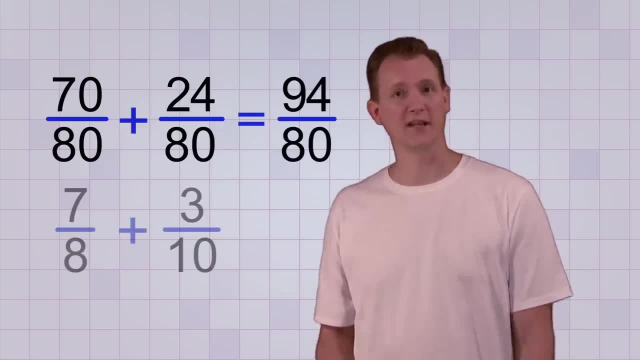 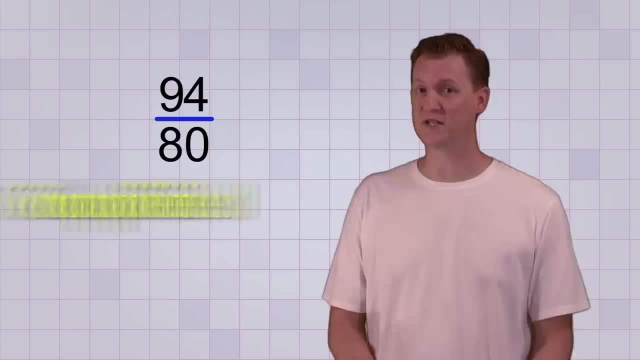 So 7 over 8 plus 3 over 10 equals 94 over 80.. Some of you see that this answer could be simplified. Be sure to check out our videos on mixed numbers and simplifying fractions to see how you could do that for your final answer.